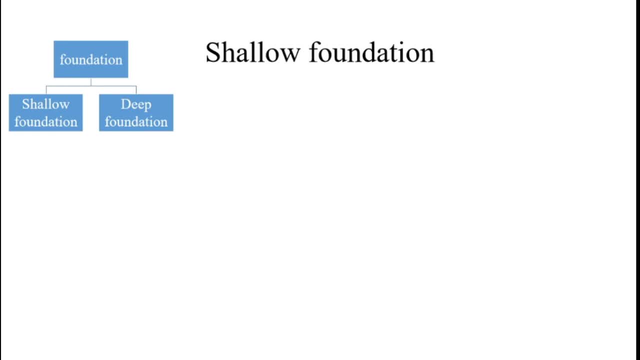 Hello everyone, welcome back to the part 1 of Shallow Foundation. So this is my second attempt of making this video. In the first attempt I forgot that I was recording or not, So I didn't check it. and it turns out I taught the entire lecture and I didn't put the recording on. So just remember, kids, bad thing happens to good people all the time. You should not worry about it. 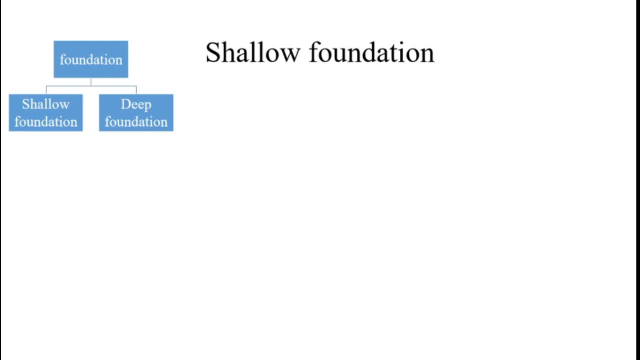 Okay, so on that lighter note, let's start with the foundation. So, basically, foundations are divided into two parts that you already know. You might have studied this in your second year, I hope so. If not, then don't worry about it. So Shallow Foundation are divided into two parts: Shallow Foundation and Deep Foundation. 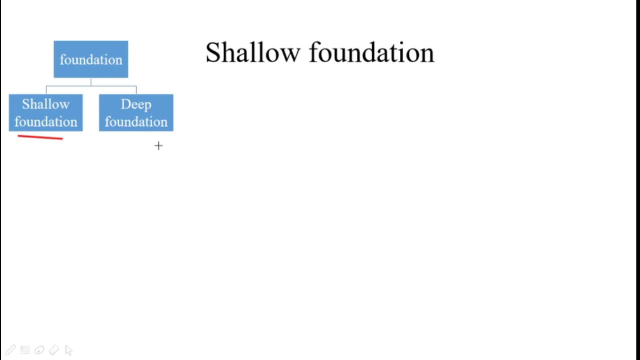 So in this chapter what we are going to see- how to determine how to design a Shallow Foundation. If and when you design a Shallow Foundation, you are going to see how to design a Shallow Foundation, Whether a particular soil will be able to carry that load of that foundation or not. that we are going to see in this chapter. So Shallow Foundation is probably the most important chapter in the Geodeck 1 and 2 because everything that we are studying we are studying to calculate the bearing capacity of the foundation. 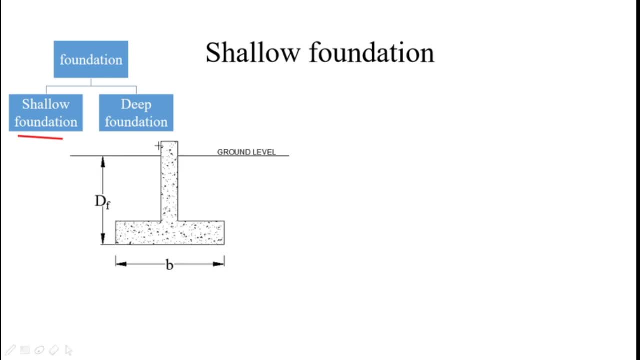 Okay. so next thing, we must know how we categorize a foundation, On what basis, the primary basis of dividing a foundation into shallow or deep, based upon these two parameters, that is, depth of foundation from ground level and width of foundation at the base. 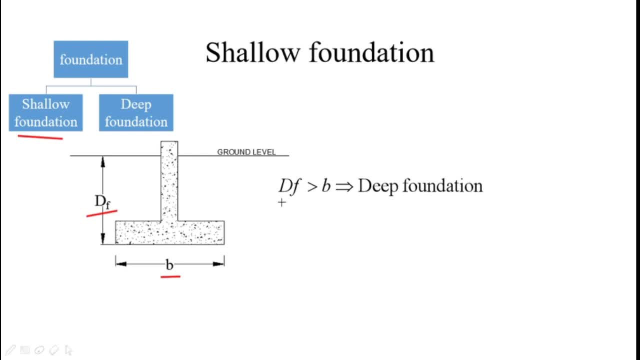 So if your Df is greater than the value of B, those foundations are categorized as deep foundation And, contrary to that, if Df is less than B, then those foundations are categorized as deep foundation. So if your Df is greater than the value of B, then those foundations are categorized as deep foundation. 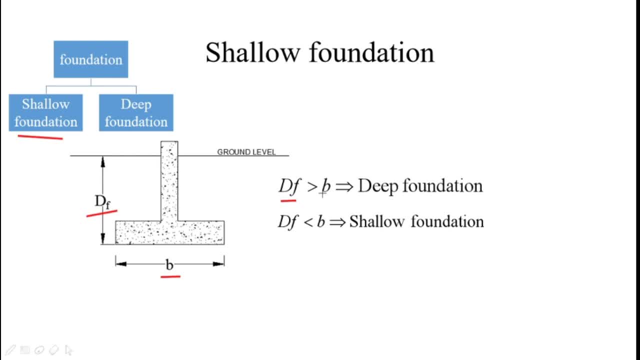 So if your Df is greater than the value of B, then those foundations are categorized as shallow foundation. Okay, so one of the few examples of deep foundations are pile foundation and casein, And other one is shallow foundations are usually footings raft. those are also called as mats. 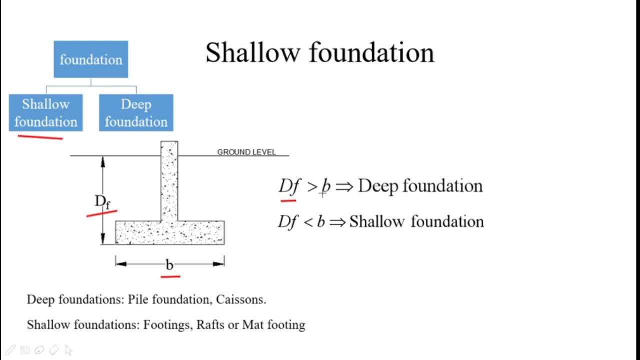 Usually, we use shallow foundation when the hard strata is available near to the ground level, And deep foundations are used when hard strata is not available near to the ground level. Okay, so one of the few examples of deep foundations are pile foundation and casein. 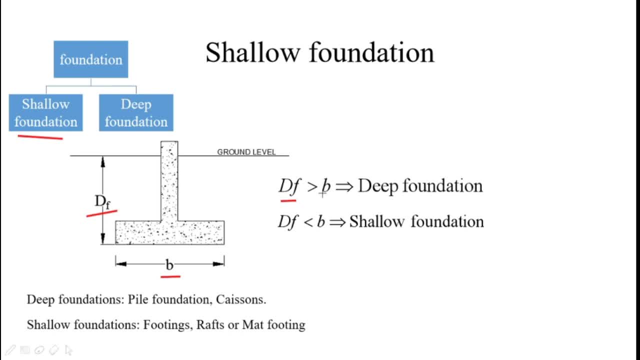 to the ground level. also, in case of a bridges or any other structure or, let's say, a very high building. in those cases you have a very huge amount of load coming on the foundation and you cannot build a shallow foundation. if you do that, it will burst into, like it will burst suddenly. 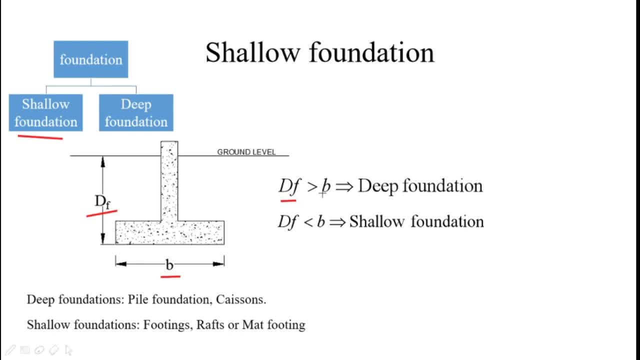 so you need to create a deep foundation in two cases. case number one: hard stata is not available near the ground level. case number two: the loads which are coming onto your foundation are very large, so in these two cases we build a shallow foundation. these cations are like a very old. 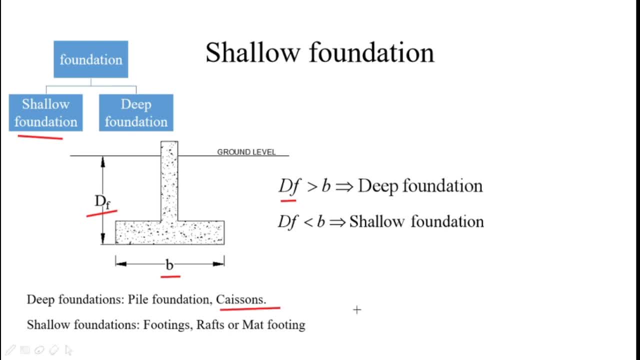 primitive technology that we don't use nowadays. the reason is cations are usually like in older days. what used to happen when a bridge foundation needs to be built. what we used to do is: let's say: this is your water level and you need to build a shallow foundation and you need to build a. 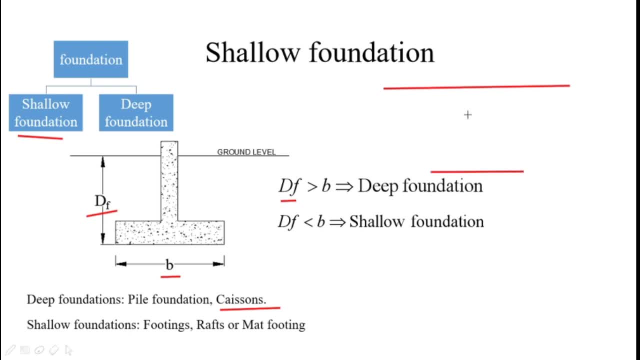 foundation over here. so what people used to do is they used to create airtight container like this. it will be like this and it was airtight so that water cannot enter inside and you have to send the people inside over here. and these people used to dig the ground. once the ground 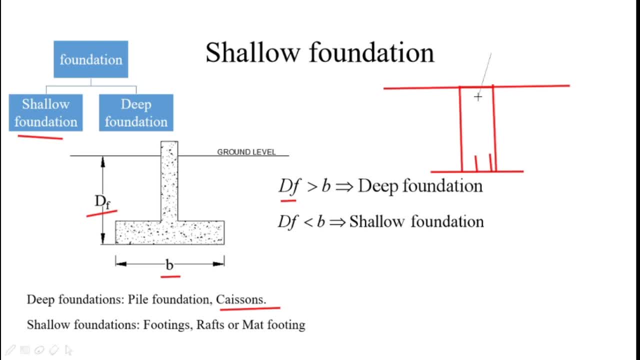 is properly dug, then you pour the concrete over here from here. but as these cations are right here, you need to build a foundation over here. so what people used to do is they used to pneumatically sealed airtight. a lot of people used to die because of that, because of the there. 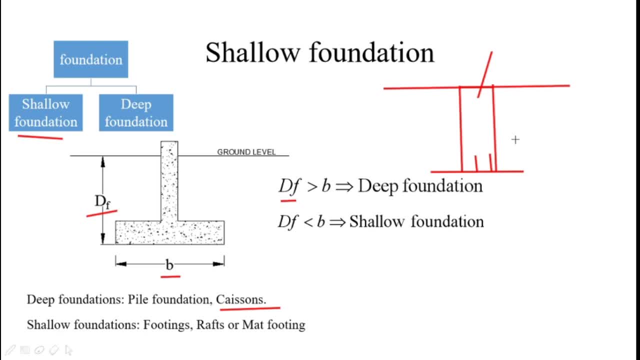 is a one sickness with sickness that used to happen inside the people. we used to call it that sickness as a deep compression sickness. so to avoid those depth feet- death- we don't nowadays use cations, we just go for the pile foundation. next one classification of foundation for shallow. 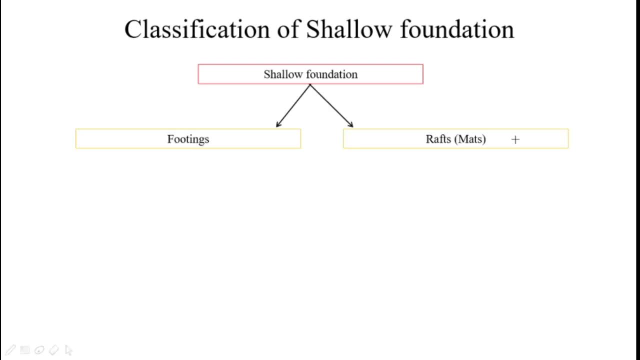 foundation is called the shallow foundation. the shallow foundation is the foundation which is called the shallow foundation. shallow foundation are broadly classified into two categories. first is the footing. other one is raft. footing are generally used when the soil which you have has a very good bearing capacity and it can withstand the load. if you build a very small, 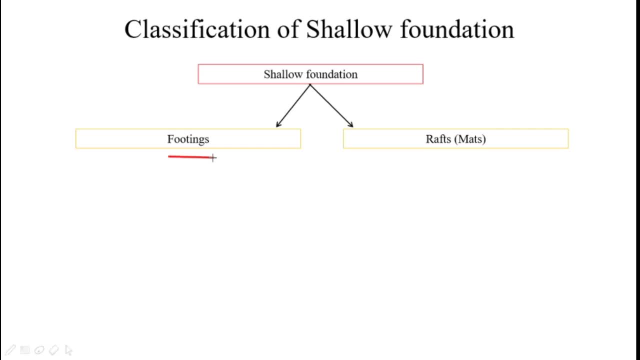 foundation. if the area of foundation is very less still, your soil is withstanding that load. then you may build a footing and raft are built in case of a very weak soil, let's say in case of a black cotton soil or a clay soil. if you build a footing on that soil, what will happen? footings are very smaller. 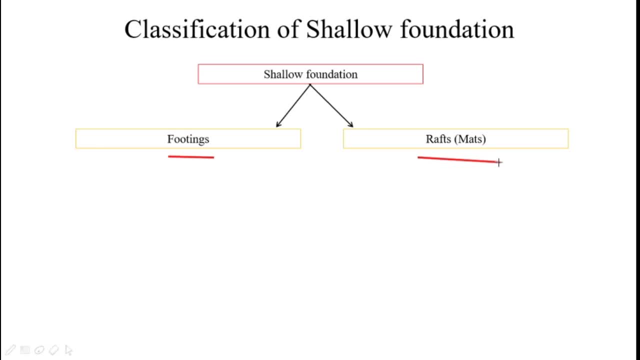 area as compared with the raft. so footing will punch inside your soil and that will fail your structure. so raft are just like mats, like that we use onto our floors, so they spread the your stresses to a quite a large area. then again, footings for our purposes are classified into three categories. 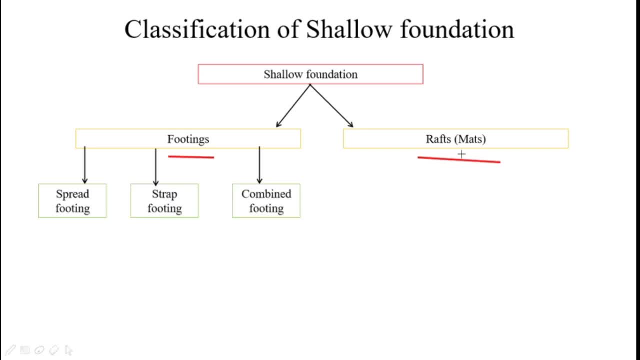 strap footing and combined footing will not go into detail of each one of this. we'll just see one more classification of footing based upon shape. spread footing are classified into square footing, circular footing and rectangular footing. the shape of the footing depends upon shape of column, if your 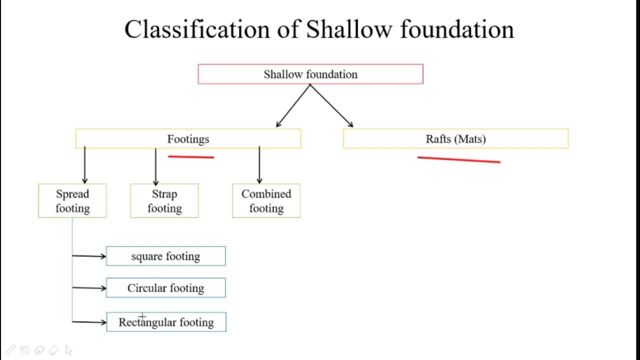 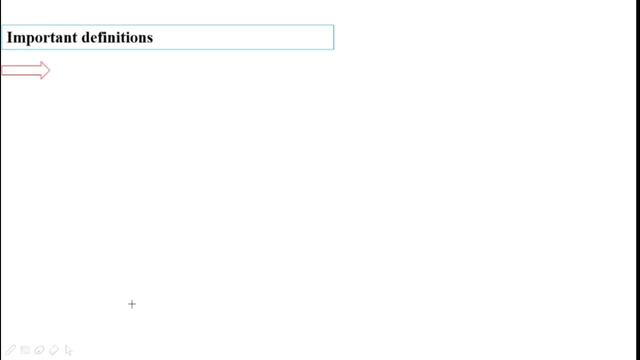 column is square, it is better to have a square footing. similarly, if your column is circular, it's better to have a circular footing. next, some important definition. these definition comes into the exam and these are also important in order for you to solve the numerical. so you must remember this definition by heart. so the first definition is: 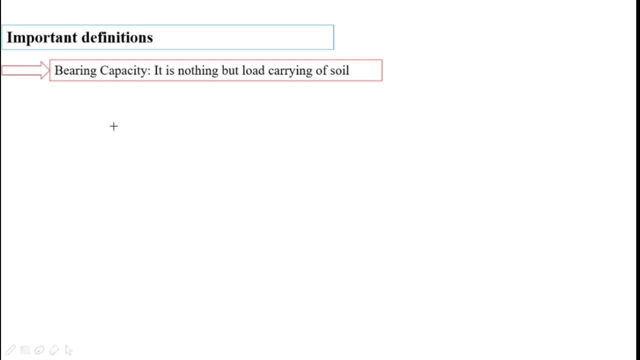 bearing capacity. bearing capacity is nothing but the load carrying capacity of soil, just like a concrete. let's say a concrete has a compressive strength of 20, it means it can carry 20 Newton per mm square of the load. similarly, if you say a particular concrete as a bearing capacity- soil. 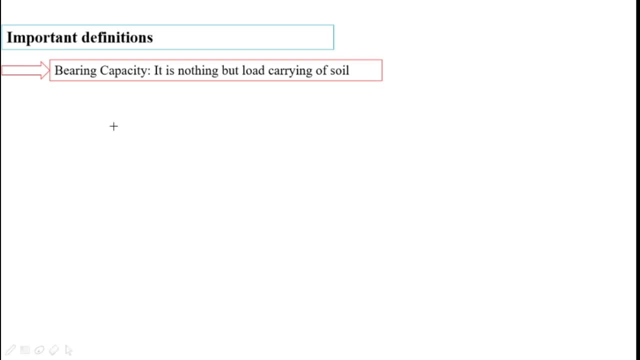 it means it can carry 180 kilo Newton per meter square. okay, so that's what the bearing capacity is. but this definition- first definition- is not very useful. it does not convey a lot of information that we had- you will see later on. so the second definition, which is very important, is ultimate. 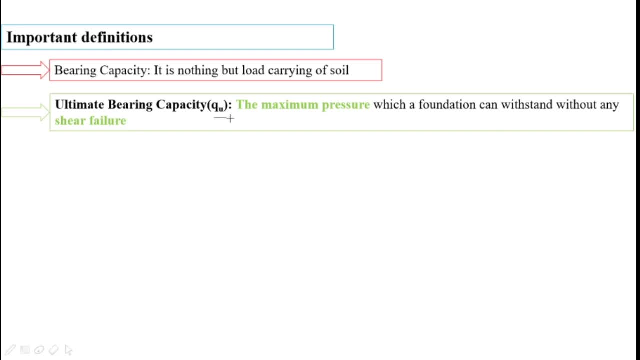 bearing capacity, which is denoted by symbol Q- you, or in some book it is called as a Q: ultimate. okay, so the word ultimate, these. what you should know is that the load carrying capacity of the soil is maximum, so the word ultimate means maximum. so the ultimate bearing capacity can also be called as a. 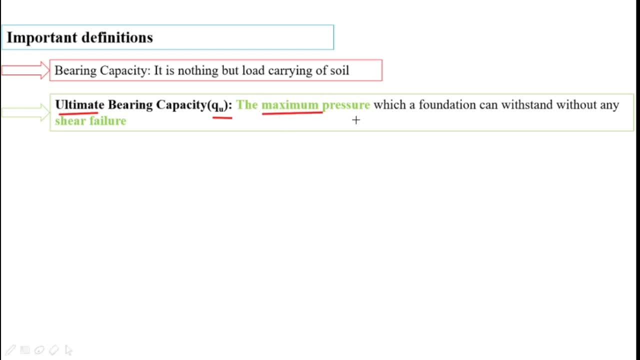 maximum bearing capacity, so the maximum pressure which a soil can withstand without any shear failure. now, in terms of soil, we do not measure its strength in compressive strength, compressive stress or in terms of a tensile stress. why? because, first thing, it is a tensile stress. 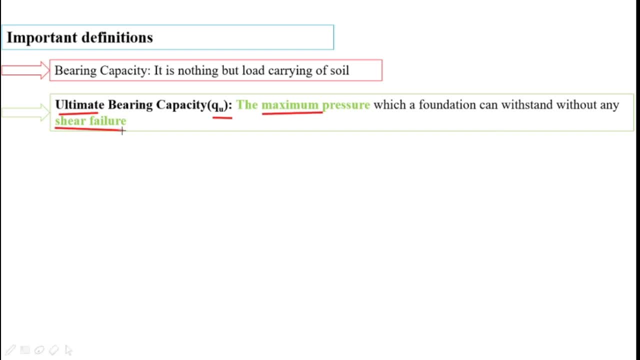 Soil does not have a lot of tensile strength, so we don't measure it. Compressive strength is very difficult to measure for the soil You need to create a sample and it does not give you very accurate idea. So to understand capacity of soil, shear strength is the probably best criteria, and that is. 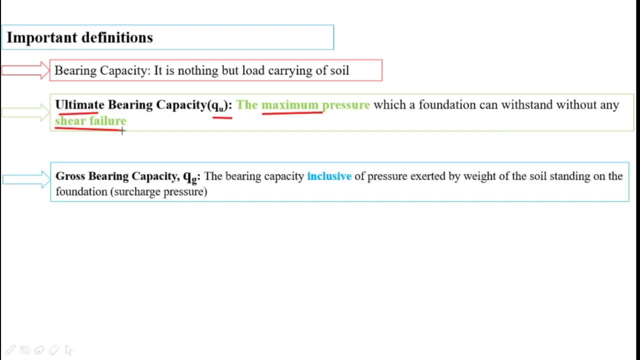 what we use. Next one is gross bearing capacity. As I said, pay attention to the word. Gross means collection of everything, So the gross bearing capacity is a bearing capacity which includes pressure exerted by the weight of soil standing on the top of the foundation. 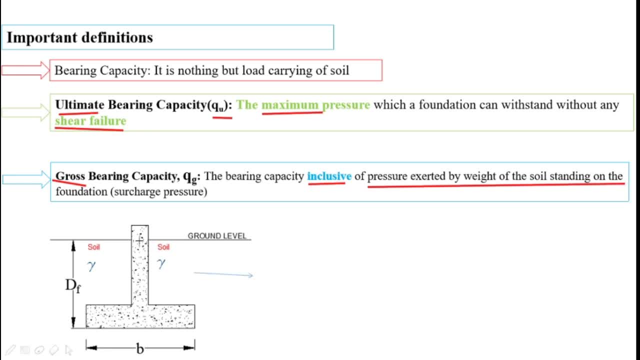 What does it mean? It means that this footing is here, This footing. when we construct this footing, we remove this much of part, then we construct the footing And after the construction foundation is done, we place the soil once again. So this soil, which is placed in this region or in this region, exerts its own pressure. 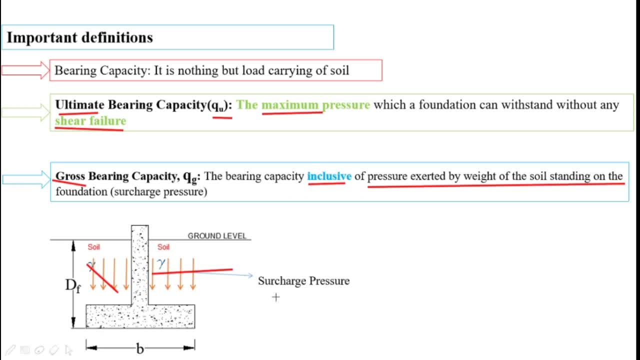 That pressure is called as a surcharge pressure- that you see over here- And surcharge pressure is nothing but weight of the soil which is standing on the footing. So, as it is a weight, you can calculate the surcharge pressure, which is denoted by symbol. 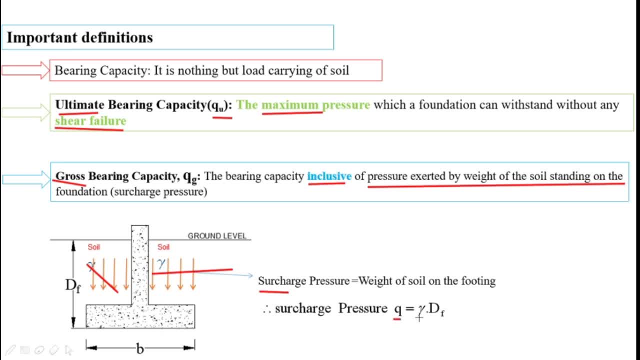 QU By formula of weight. Now you will say formula of weight is: unit equals to unit weight multiplied by the volume. But remember, we are dealing in 2D. So in 2D you don't have area concept of area, you have only concept of height. 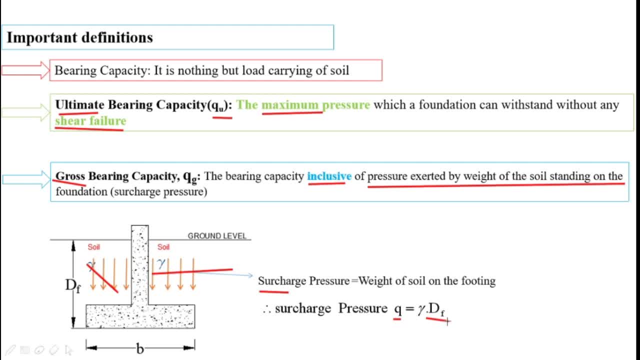 So basically your surcharge pressure QU becomes gamma multiplied by this TF. Now in some books or some papers or some theories you will see DF is taken Till this height or sometime DF is taken at this height. If you take the DF till this place, till the bottom, you will be much more safer because 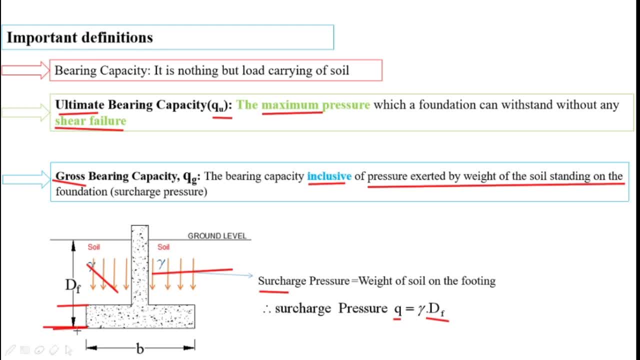 you are assuming more weight over here. That's why, for all intensive purposes, for as far as our syllabus is concerned, we will measure the DF from this point till this point. In some books, you will find out, DF is also measured till this point. 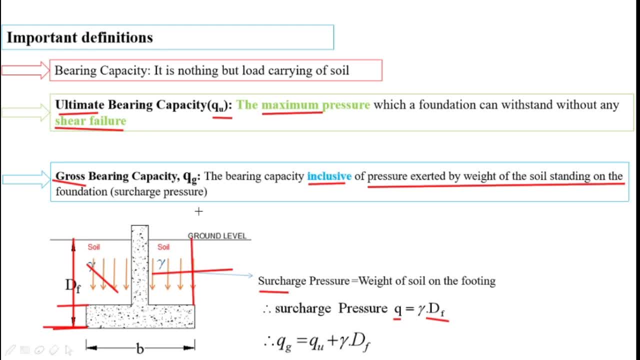 Okay, Next, By the definition, this QG, that is, cross bearing capacity, is equals to this ultimate bearing capacity which we have just determined. that is maximum bearing capacity plus this gamma DF, that is weight of this soil over here. Next definition: net ultimate bearing capacity. 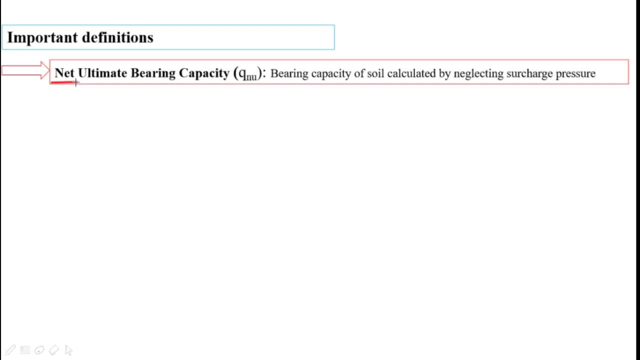 Now the word net. Net means whatever is affecting whatever is affecting your structure. So what is affecting your structure? What does impact net? So net bearing capacity of soil is calculated by neglecting the surcharge pressure. In gross, what we had done is let me show you we had added this gamma DF. 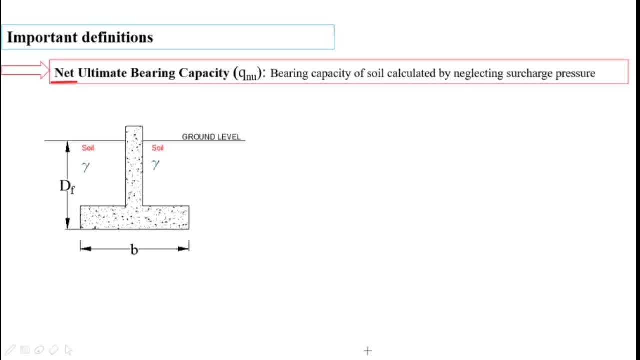 In net ultimate bearing capacity. what we do is we just subtract this gamma DF. So from your QU that is ultimate bearing capacity. if you subtract this weight, that is gamma DF, you get a net ultimate bearing capacity, which is denoted by symbol QNU. 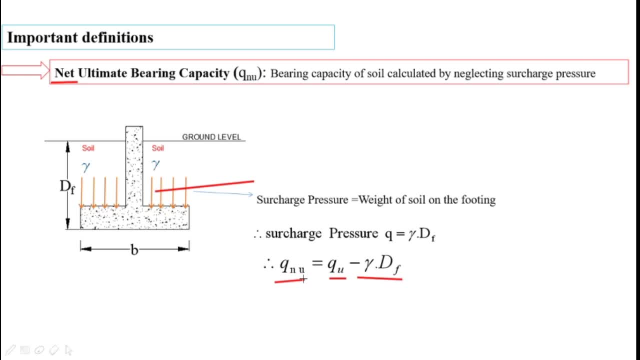 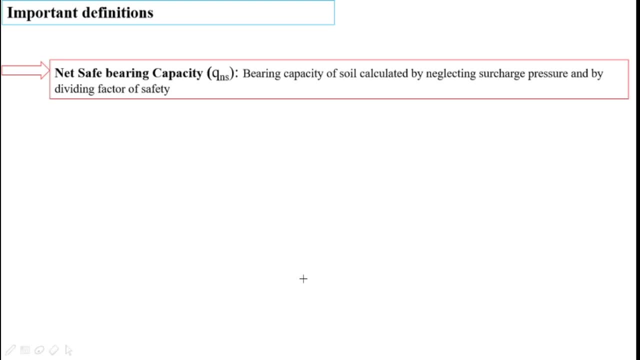 Net stand for N. stand for net. U stand for ultimate. Next definition: net safe bearing capacity. Now what we have added over here. another word: safe. So how does a thing become safe that you need to understand first. Let's say a concrete cube has a strength of 20 Newton per mm square. 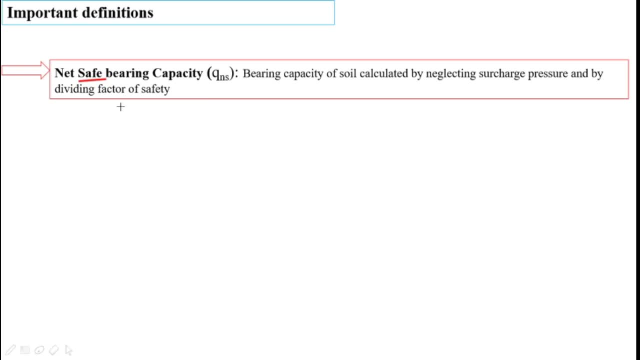 But when I am applying this strength of 20 Newton per mm square, But when I am applying the load, let's say I create a column using that concrete. So when I am applying the load on the column I will not apply. the load equals to the carrying. 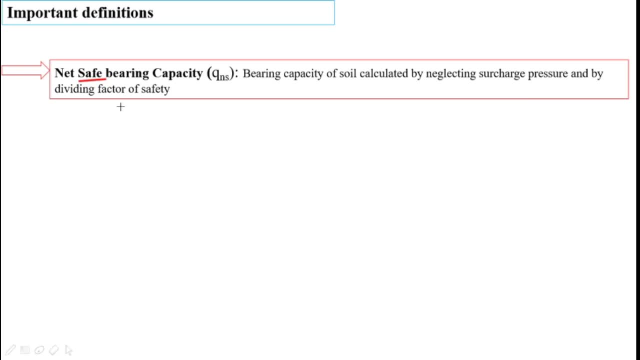 capacity of that concrete. If I do that, the structure will fail. So what I will do? I will just apply the 50% of the load. So what does it basically mean? Now, your column concrete will remain safe. Why? it is same. 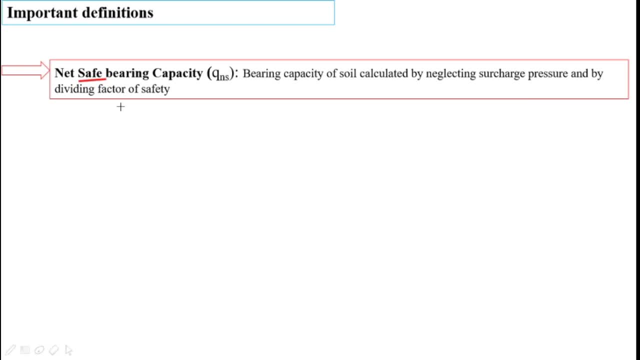 Because you have applied a factor of safety of 2. That is, you have only applied 50%. That is what the net safe bearing capacity is. So what you will do is you will just calculate your net safe bearing capacity, that is, Q and U, and then you will divide it by factor of safety. 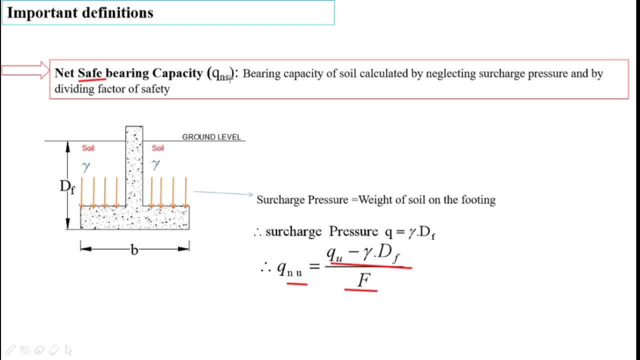 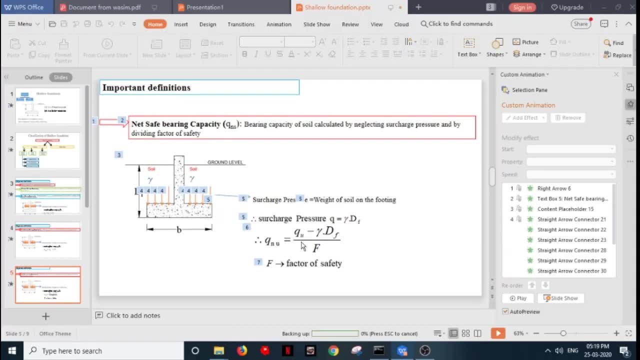 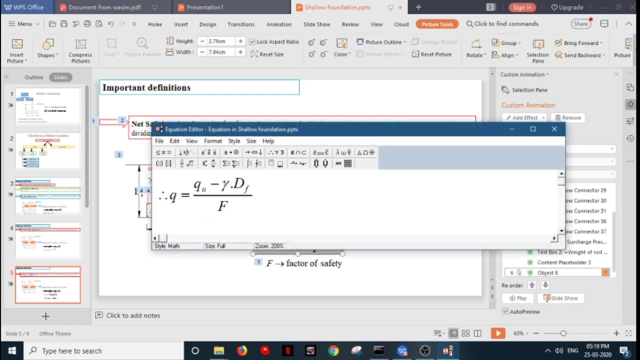 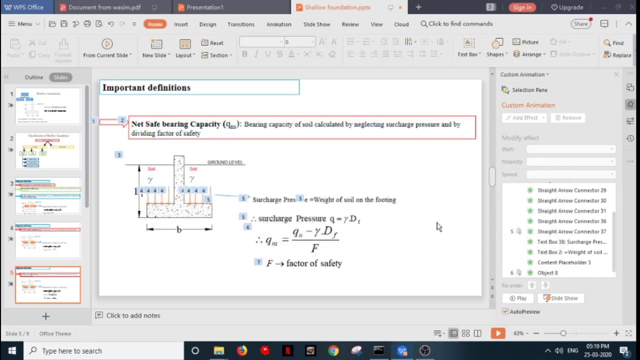 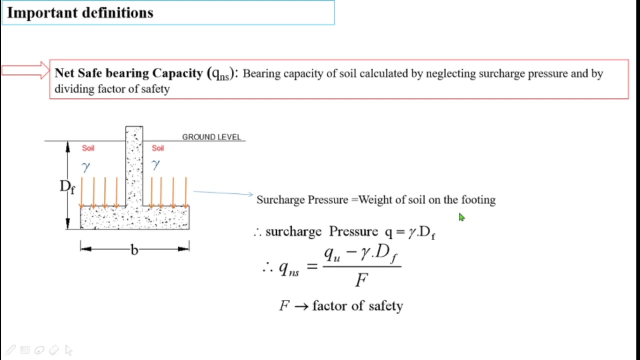 So you will get the value Q and S. Sorry, this should be Q and S. Let me correct it. discard this value. this symbol should be Q and S. Q and S. Okay, Cool Chalo. next, Net safe bearing capacity. the only thing that we did is we divided it by factor of. 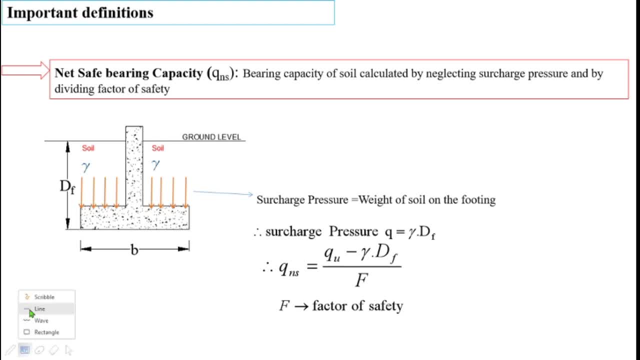 safety. Okay, Usually in case of like- let's say concrete, you get factor of safety around, let's say 1.5, and in case of steel it is 1.15.. If you compare steel and concrete, the factor of safety for steel is less. 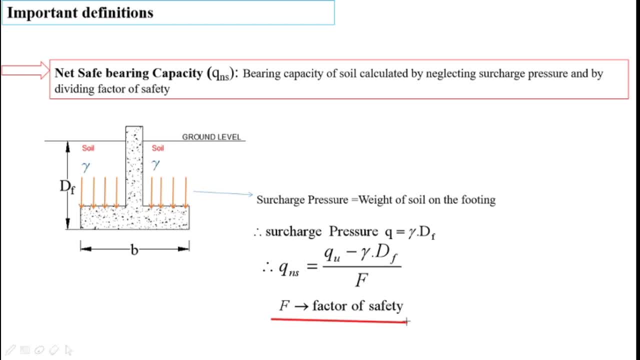 Because we are more certain, we are more knowledgeable about steel as compared with concrete. But when you come to soil, which is very rational behavior, soil does not show very consistent behavior. In summer season it will show different behavior. In winter season it will have different property. 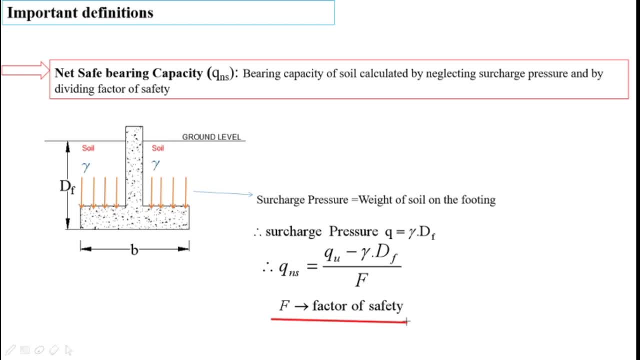 In rainy season it will have totally different property, So we are not certain how the soil behave. So that is why, when you see the factor of safety, In case of soil, that factor of safety is like 2.5 or 3.. 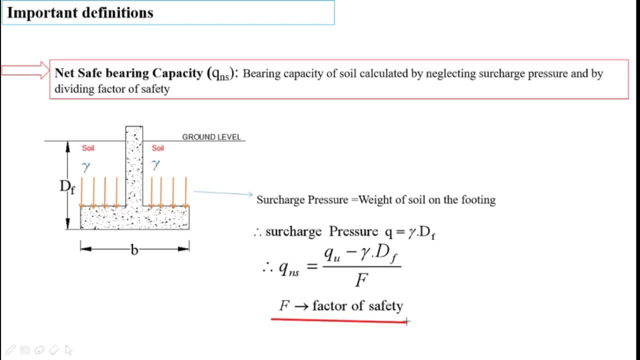 Like in concrete we have 1.5, but in soil it is almost 3,, 3.5, or in some important structure, let's say if you are building a nuclear component or a nuclear power plant. In those cases factor of safety even go to 4 or 5.. 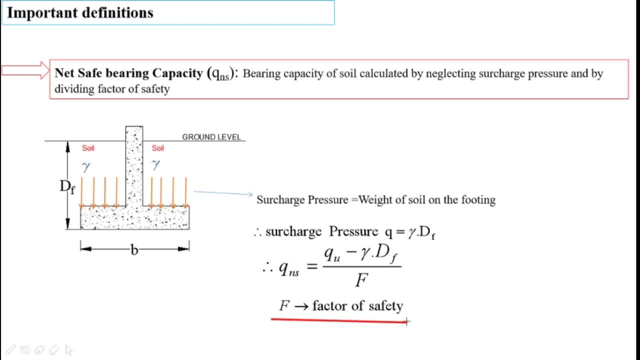 That's why you see that important structure have a very big foundation, Just like a dam. You don't want your dam to break. If it breaks it will cause lot of damage. So in those cases you use higher factor of safety. But in our case, in case of a foundation, or in case of a shallow foundation or deep foundation, 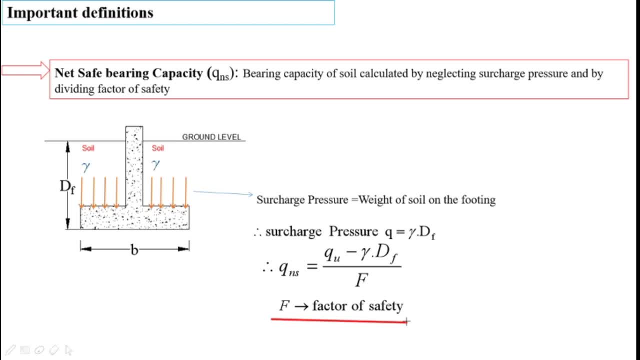 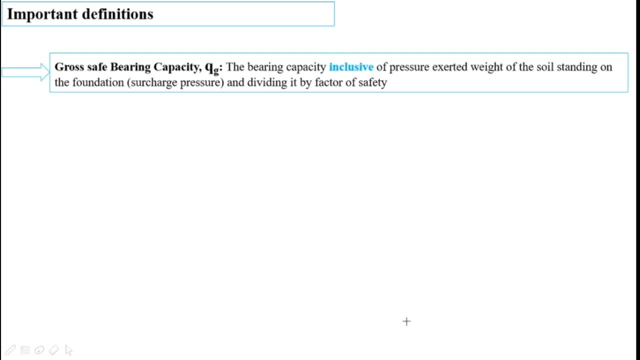 usually the factor of safety ranges from 2 to 3.. Now, next is cross safe bearing capacity. As explained earlier, the only thing that we will do over here is we will calculate cross safe bearing capacity. cross bearing capacity, that is QG. 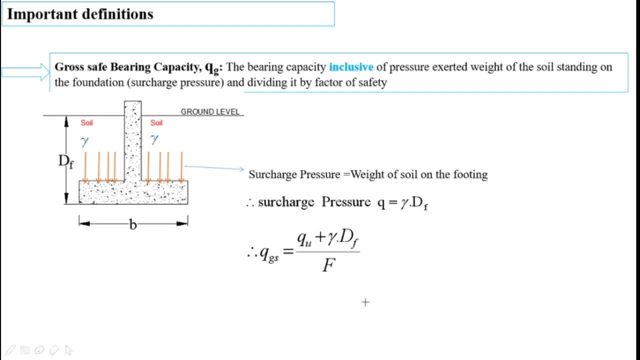 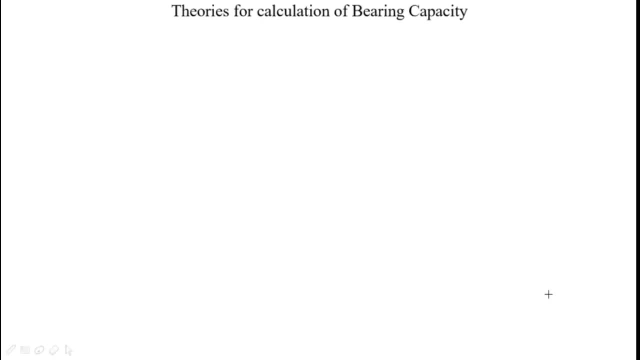 And then we will divide it by QG, And then we will divide it by QG, And then we will divide it by factor of safety F. you will get a cross safe bearing capacity. That's it. These are like. these few definitions that you have seen so far are very important. 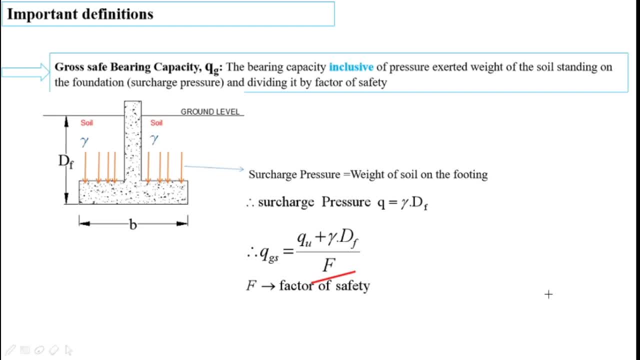 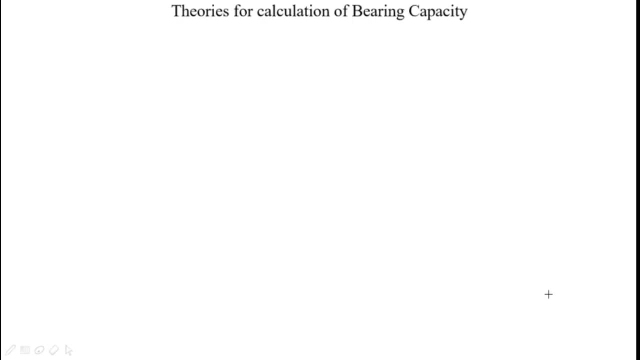 Please remember them. I will also give you an assignment in which you have to write down all these definitions. Okay enough. Next, some theories that are basically used to calculate the bearing capacity. The first theory, which was given by Rankine, Like it's probably one of the oldest theory that exist in geotechnical engineering, 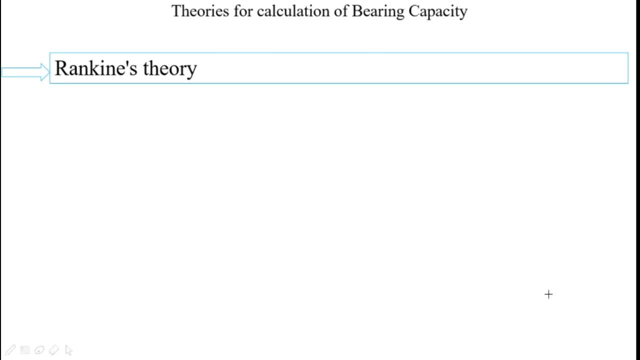 Rankine's theory is very outdated. Nobody use it nowadays, But it is important gate point of view that that's why you should study it if you are preparing for gate. Next one is Prandtl's theory. This, this name, Prandtl, you might have already heard from fluid mechanics. 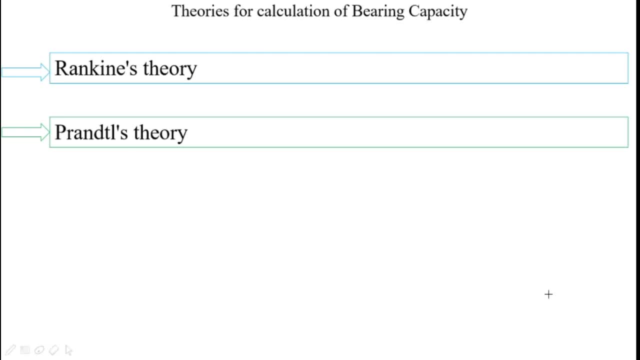 In, I think, turbulent flow. you have seen Prandtl mixing length. the same concept is also used to calculate Baring capacity. Again, these two theories, that is, Rankine's theory and Prandtl's theory, are not part of our syllabus. 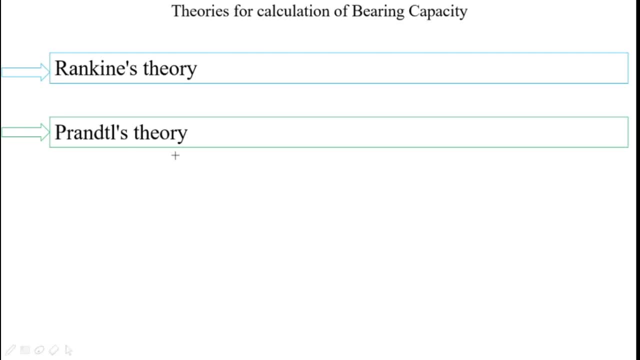 So we will not discuss that in detail. The next theory, which is Terzaghi's theory: The reason why Terzaghi is called as a father of soil mechanics is because he gave us this theory of bearing capacity. That we will study in detail. 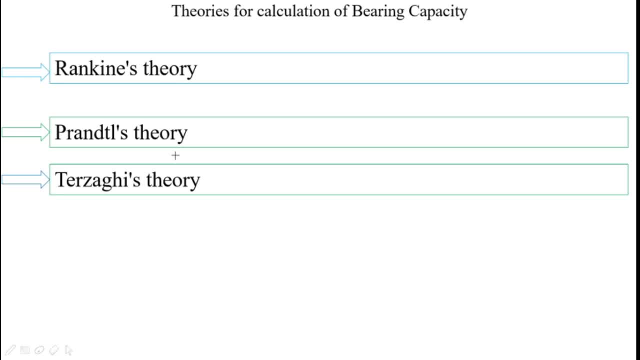 It is part of our syllabus. Next theory, which is Meyerhof's theory. Again, this theory is directly not part of our syllabus, But the theory which is part of our syllabus IS code method based upon the Meyerhof's theory. So we will see some aspect of Meyerhof's theory also. 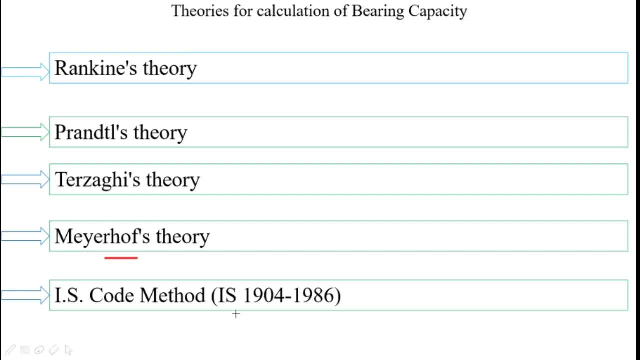 Okay. so everyone should download this code because this code will be very important in studying this IS code method. So when we will solve the numerical on, let's say, in part number 6 or 7, we will solve this numerical on IS code method, Then I will give you the link to download this code. 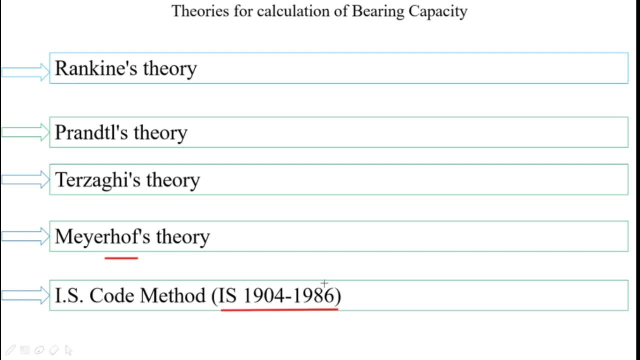 That is IS-1904-1986.. It was revised in 1986.. Since then, nobody thought of revising it. We definitely need some revision on that IS code also. Okay, so, as I said, IS code is combination of Meyerhof's theory and Terzaghi's theory. 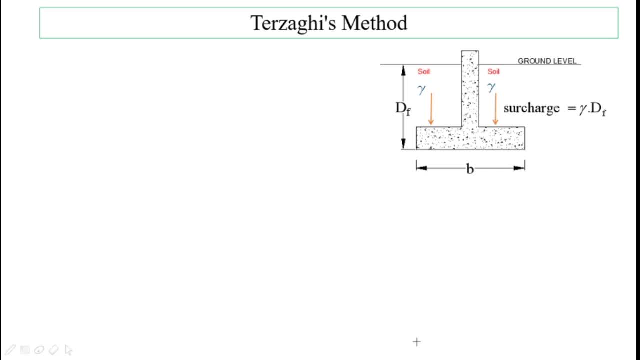 So we will start with Terzaghi's theory. We have a footing over here at a depth gamma df, we have sarchad, which is equals to q, equals to unit weight- Okay, Sigma, sorry, unit weight- gamma into df. So we will start with the assumptions in theory, then we will stop, then we will meet again. 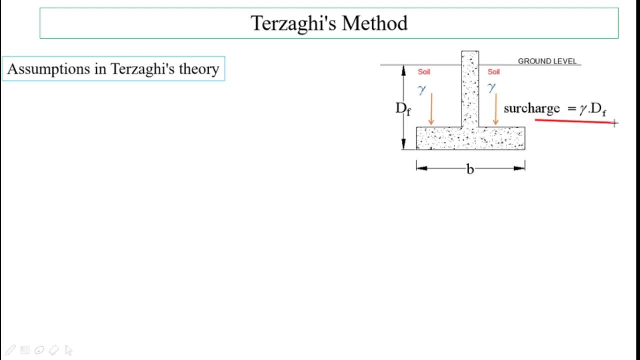 in part 2.. So the first assumption is this is: this also comes in exam lot of times. you should remember all these assumptions. There are around 10 assumptions. we will not go into all of these and those are not required. So the first assumption is: base of the strip footing. first assumption is that all the footings 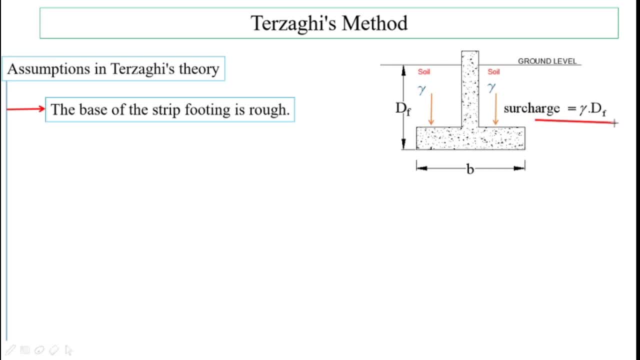 are the strip footing that I forgot to add. I don't know why That is. that should be the first one. Second assumption is that strip footing is rough, So there is a friction between this soil present over here and this concrete. That is the first assumption. second assumption of Terzaghi's theory. 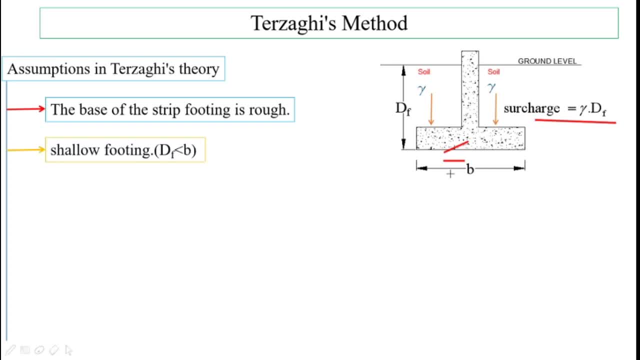 Next assumption is all the footings are shallow footing that is, df is less than b. So Terzaghi's theory: you cannot go and directly apply to pile foundation. You have to do some modification that we will see in the next chapter. Okay, 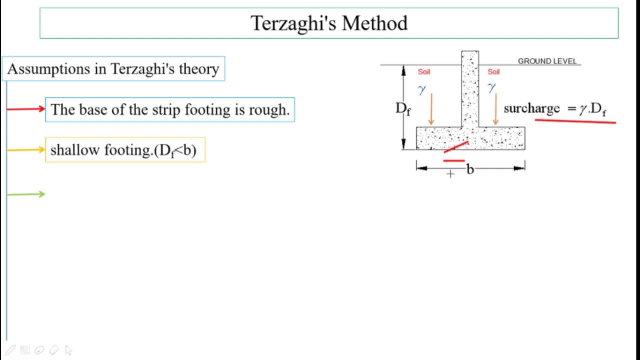 So far all the footings are in Terzaghi's method- are shallow footing. Next one, the shear strength of soil above the base of the footing, that is the soil which is present over here. Okay, there shear strength is neglected and it is replaced with a surcharge.